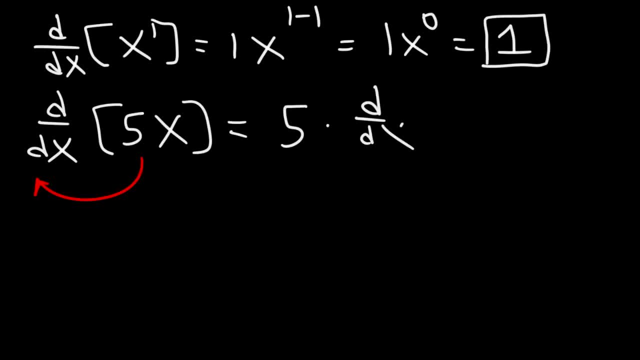 So this is the same as 5 times the derivative of x, And the derivative of x is 1, so 5 times 1 will give us 5.. The derivative of, let's say, negative 7x is simply negative, 7.. 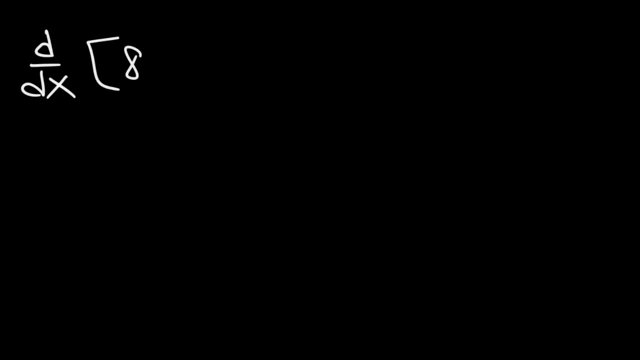 Now what about the derivative of a constant? The derivative of any constant is 0.. Now one way that you can remember that is, you can write 8 as 8 times x to the 0, because x to the 0 is 1.. 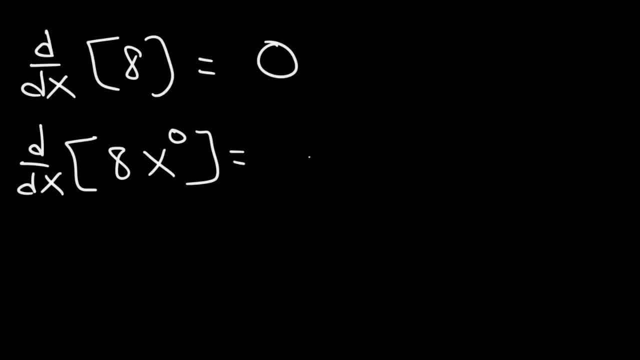 And so these two, they're the same. So this is 8 times the derivative of x raised to the 0.. And using the power rule, it's going to be 0x raised to the 0 minus 1.. And 0 times anything is 0.. 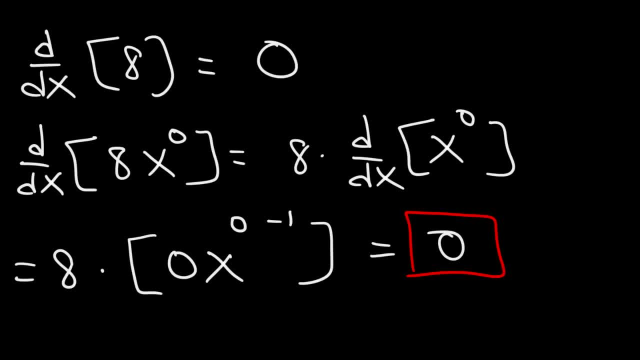 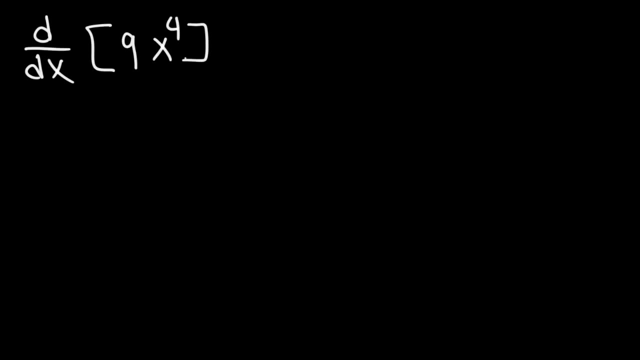 So the whole thing is just going to be 0.. So make sure you remember that The derivative of any constant is always equal to 0.. Here's another one. Find the derivative of 9x to the 4th and also 7x to the 4th. 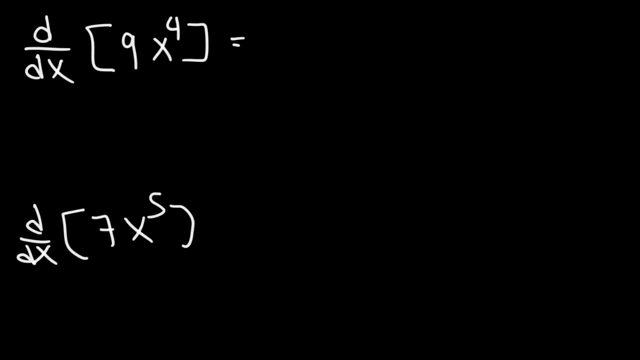 So this is going to be 9 times the derivative of x to the 4th, which is 4x raised to the 4 minus 1, or 4x cubed, And then you just got to multiply 9 times 4.. 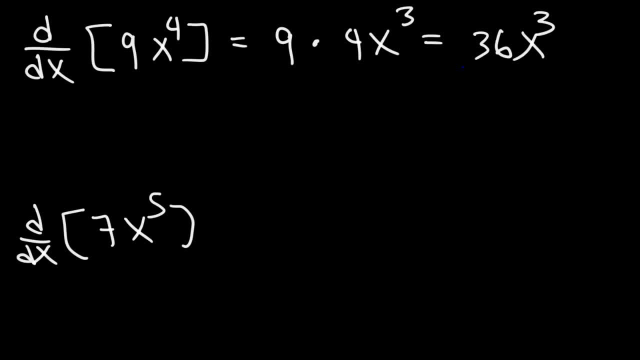 So the answer is going to be 36x to the 3rd power. For the next one, it's going to be 7 times the derivative of x to the 4th, Which is 5x to the 4th power. 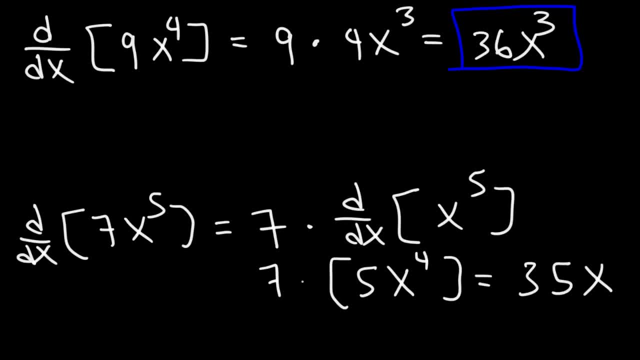 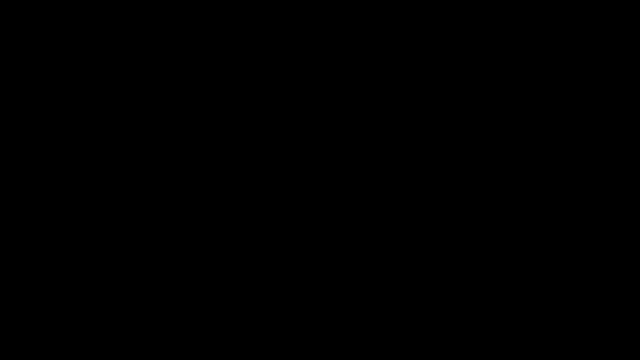 And then 7 times 5, that's 35. So you get 35x raised to the 4th power. Now what about the derivative of, let's say, a polynomial function: 4x to the 5th plus 7x cubed? 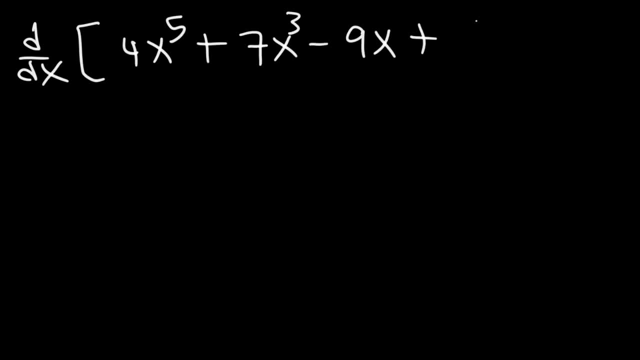 minus 9x to the 4th power, x plus 5.. Go ahead and try that. So the derivative of x to the 5th is going to be 5x to the 4th power. The derivative of x cubed is 3x squared. 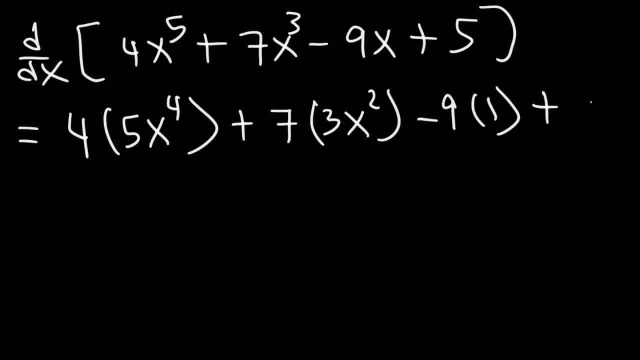 And the derivative of x is 1.. The derivative of a constant is 0. So 4 times 5 is 20.. 7 times 3 is 21.. And this is going to be it. So it's 20x to the 4th. 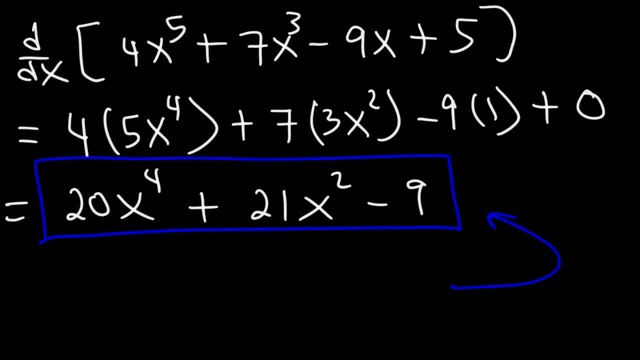 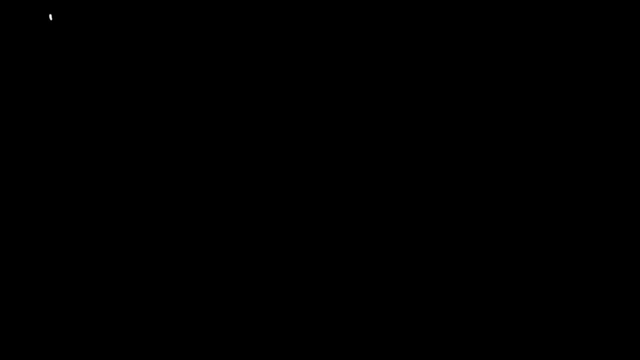 Plus 21x squared minus 9.. So you just have to differentiate each term separately. Now, what about this one? What is the derivative of the square root of x? Go ahead and try that. For this example, we need to rewrite it. 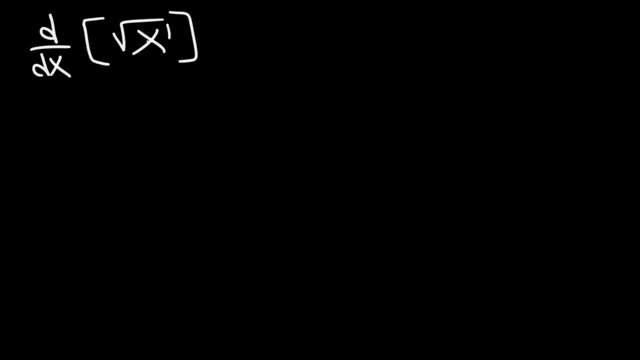 This is x raised to the 1st power, but within a square root symbol, And the index number is a 2, if you don't see a number there, And so the way you rewrite it is like this: It's going to be x to the 1 half. 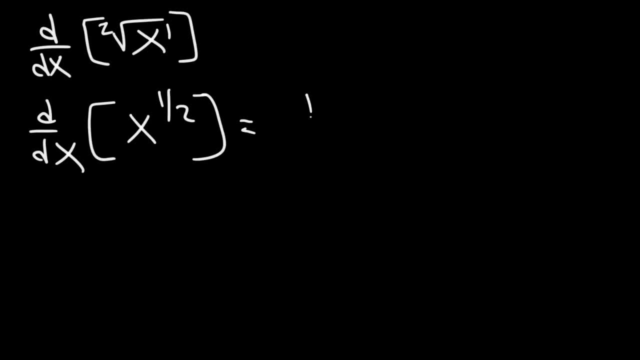 Now we can use the power rule. So it's 1 half times x raised to the 1 half minus 1.. 1 half minus 1 is the same as 1 over 2 minus 2 over 2.. 2 divided by 2 is the same as 1.. 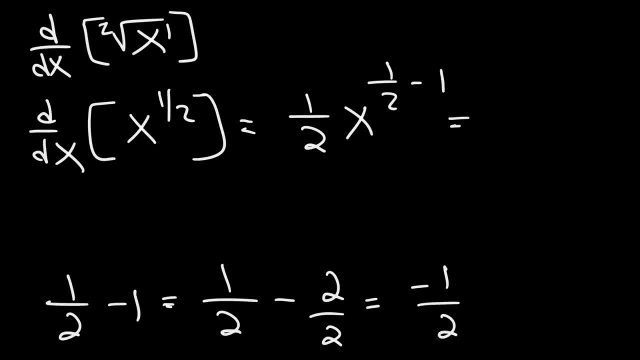 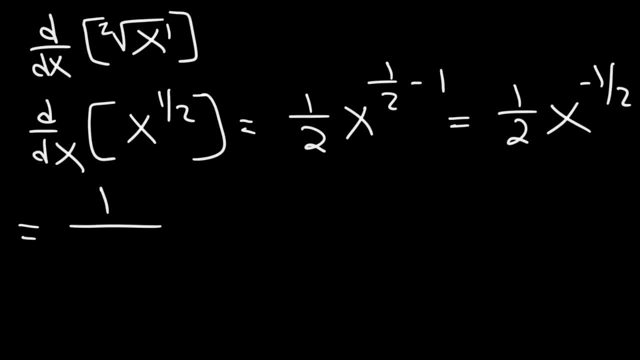 Now, whenever you have a negative exponent, you need to move the variable to the bottom of the fraction. So we're going to put x in the denominator of the fraction, So the exponent will change from negative 1 half to positive 1 half. 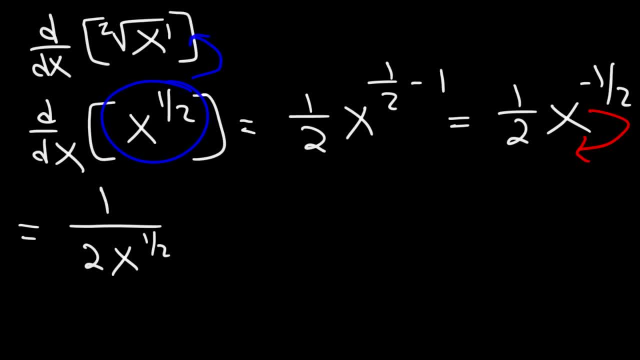 And recall that x to the 1 half is the same as the square root of x. So at this point we can replace x to the 1 half with the square root of x, And so this is the first derivative of that function. 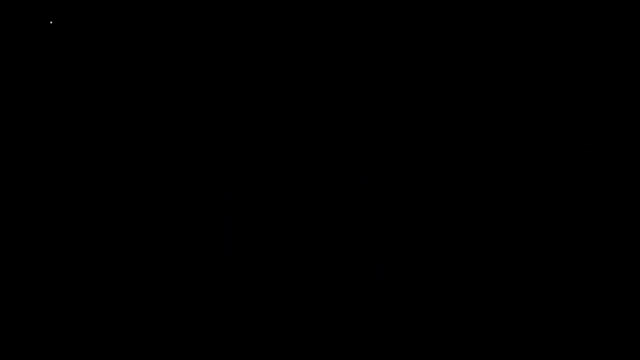 the square root of x function. Let's try another radical function. Let's use the 7th root of x to the 4th power. So the first thing we need to do is rewrite it. This is going to be x- X to the 4th power. 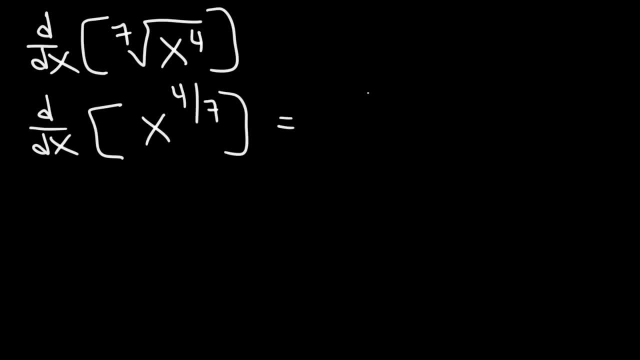 So we get 4 over 0.. So we get x to the 4th power. So we add 1 And now we can use the power rule to the power rule. So we do this by simply wingsadd x So we could use the power rule. 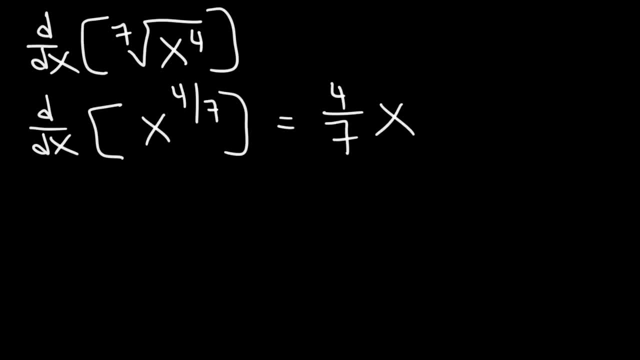 So it's 4 over 7.. 4 over 7, x raised to the 4 over 7 minus 1.. So 4 over 7 minus 1 is the sum of 4 times x to the 4 over 7 minus 1.. 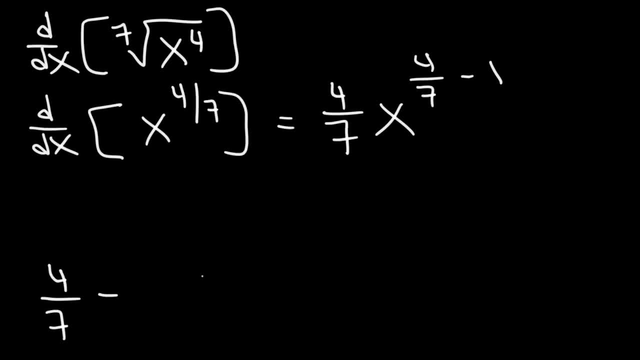 So to this we then expand the great factor into 4 over 7, minus 1,, minus 7 over 7,, which will be negative 3 over 7.. And so this is going to be 4 over 7,. 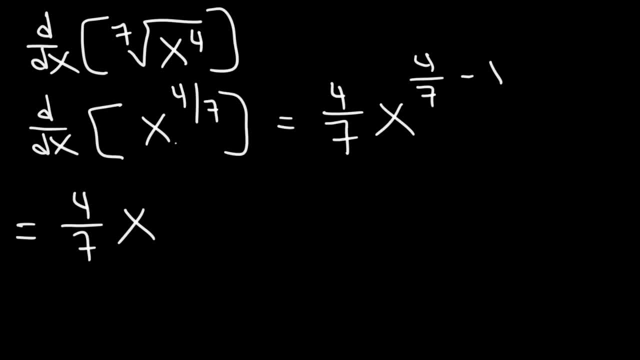 minus x to the 4 over 7, x raised to the negative, 3 over 7.. So once again we have a negative exponent, which means we need to move the variable to the bottom of the fraction. So the 4 is going to be on top, the 7 is going to. 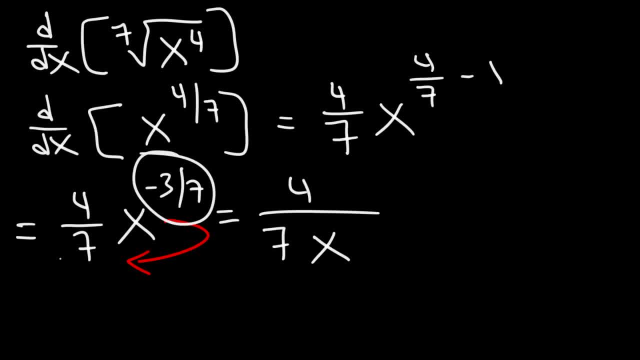 be on the bottom with the x variable and we're going to change the negative exponent to a positive exponent and then at this point we can turn it back into its radical form. So it's 4 over 7 times the 7th root of x cubed. Now, if you want to, you can rationalize the denominator, but I'm not going. 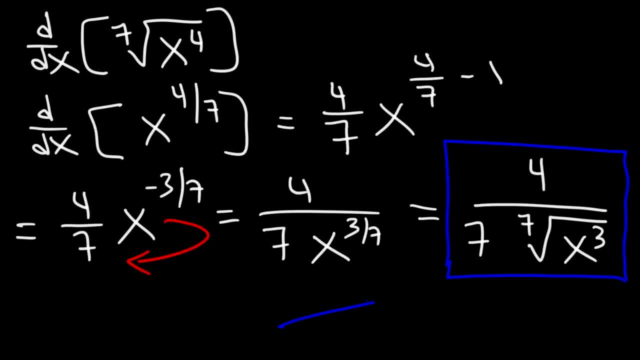 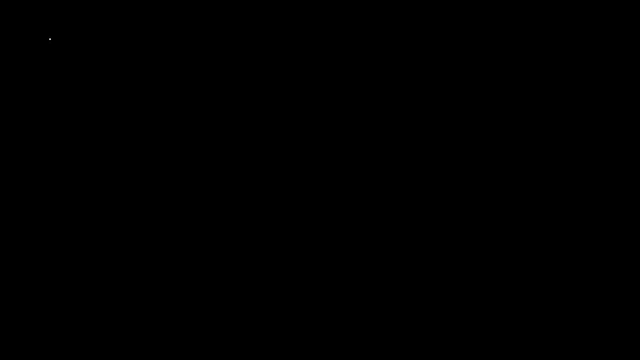 to worry about that in this example. So I'm going to leave the answer like this: and so that's how you could find the derivative of a radical function. Now, what about the derivative of a rational function like this one? What is the derivative of 1 divided by x raised to the fifth? 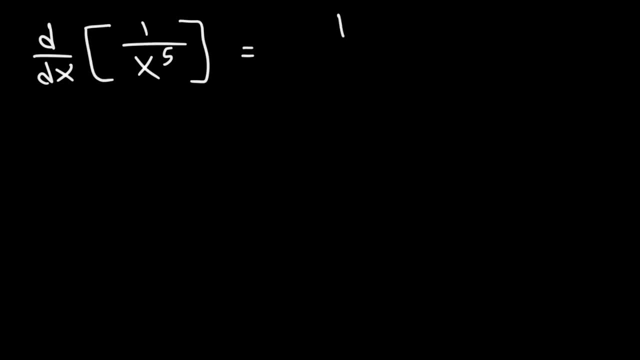 power. So once again, we need to rewrite it before we could use the power rule. So what we're going to do is we're going to take the x variable and move it to the top, and as you do so, the exponent will change sign: It's going to flip from positive 5 to negative 5.. So now we could use the power rule. 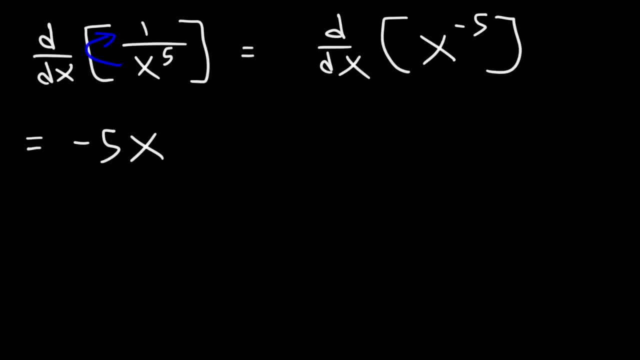 n is negative 5, so it's going to be negative 5 times x raised to the negative 5 minus 1, which is negative 5x to the negative 5.. So this is the answer, but we want to rewrite it Since we have a negative exponent. we're going to: 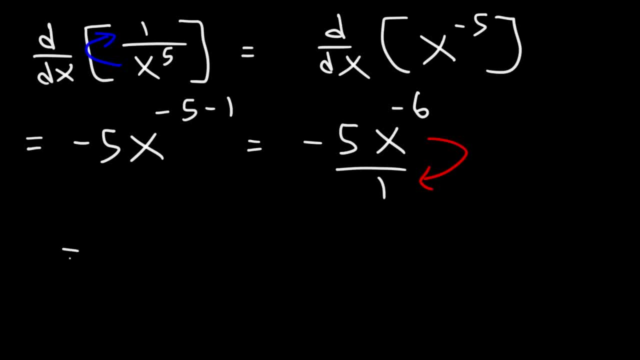 move the x variable back to the bottom. So the final answer is going to be negative: 5 over x to the sixth power, And so that's how you could find the derivative of a rational function. Now let's talk about the derivative of trigonometric functions. So here are some notes that you need. 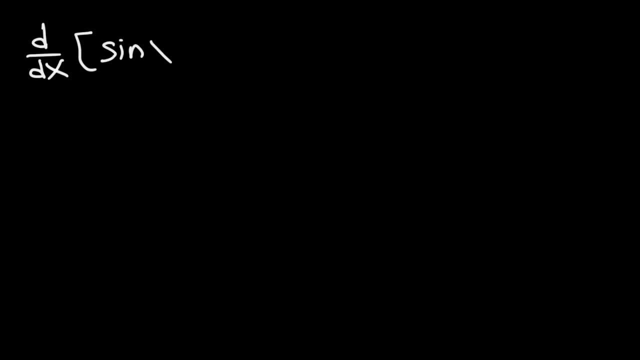 to take a look at. Take down, The derivative of sine x is cosine x And the derivative of cosine x is negative sine x. Next, you need to know the derivative of tangent x, And that's going to be secant squared. Now what do you think? 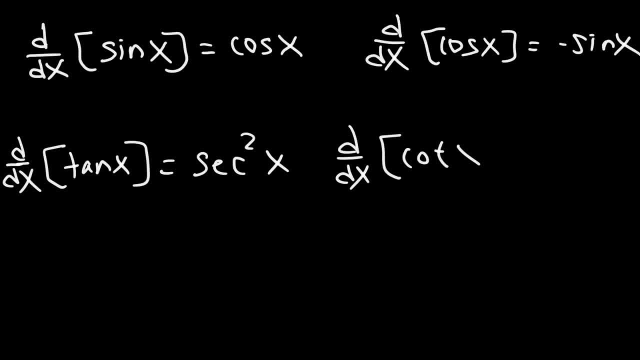 What do you think the derivative of cotangent x is equal to? It's going to be negative cosecant squared. Now the derivative of secant x is secant x, tangent x. Based on that, what do you think the derivative of cosecant x is going to be? 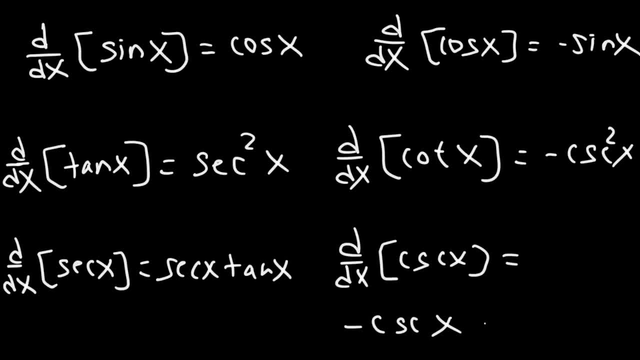 This is going to be negative. cosecant x times cotangent x And notice this pattern. So anytime you have a trig function that starts with a, c, notice that in the derivative they all have a negative sign. So that can help you to remember the derivative of the six trigonometric functions. So if you know the derivative of sine, 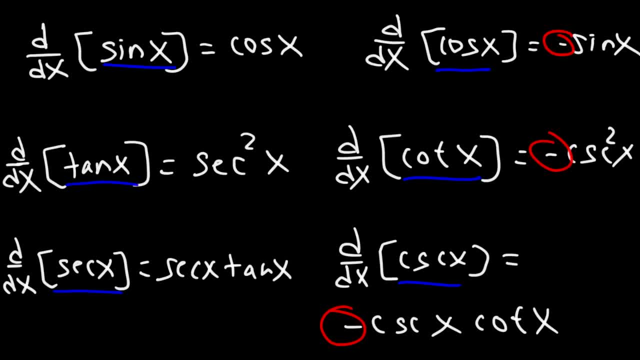 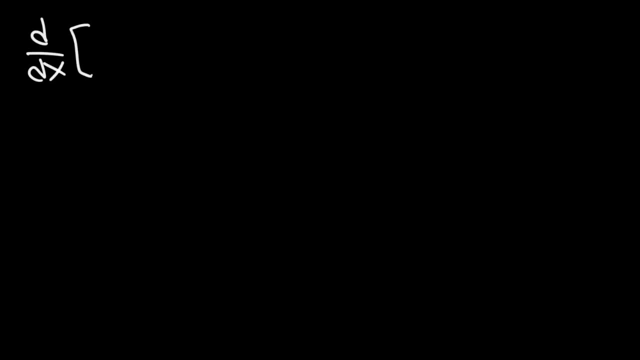 tangent and secant. you can easily figure it out. find the derivative of cosine, cotangent, cosecant, looking at the similar relationships between what you see on the left side and what you see on the right side. Now, what about this one? Find the derivative of 5 sin x minus 7. 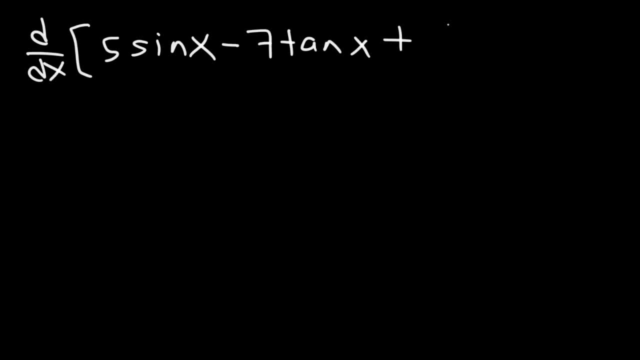 tangent x plus 4 amigos, cosecant x. So all we need to do is to differentiate each one separately. The derivative of 5 sin x is going to be 5 times the derivative of sine x, which is cosine x. Now, once you differentiate sine, next we need to. 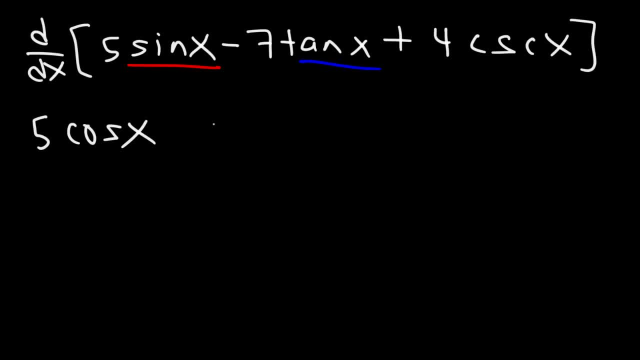 differentiate tangent, the derivative of negative 7. tan x is going to be negative 7 times secant squared. since that's the derivative of tangent And the derivative of cosecant, we set it to negative cosecant cotangent, And so this is the answer. 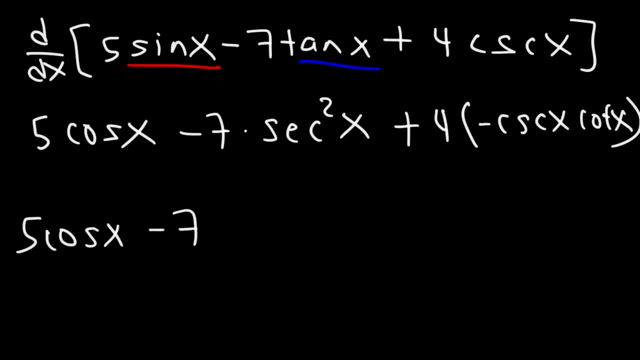 5. cosine x minus 7. secant squared x minus 4. cosecant x, cotangent x. So that's how you could find the derivative of trigonometric functions. Now let's talk about the derivatives of exponential functions involving the base e. 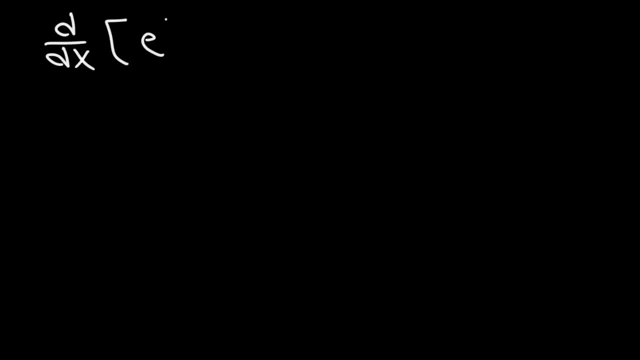 Here's a formula that you're going to find useful: The derivative of e to the u, where u is a function of x, is e to the u times u prime. So for instance, let's say, if we want to find the derivative of e to the x, 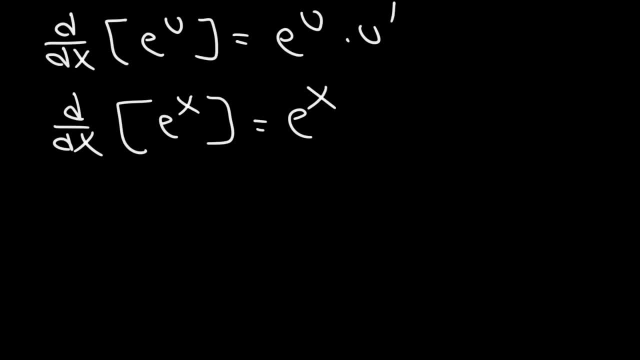 It's going to be e to the x. so u is x times the derivative of x, which is 1.. So the answer is just e to the x. Based on that, what is the derivative of e to the 7x? 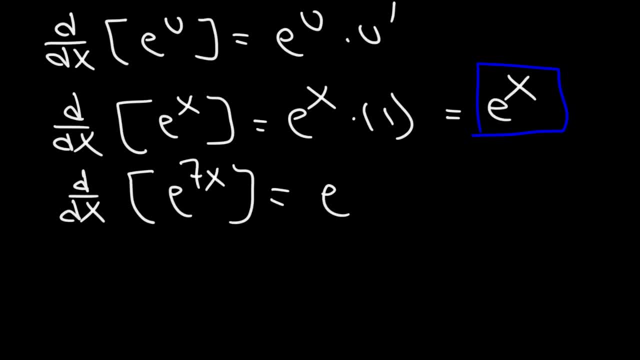 Go ahead and try that. So it's going to be e to the 7x times the derivative of 7x, which is 7.. So it's 7e, So it's 7e to the 7x. Let's work on some more examples. 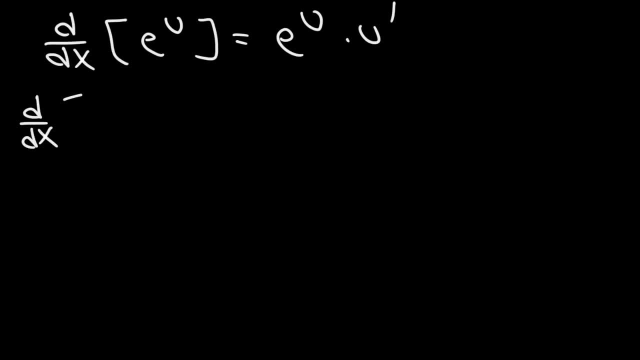 Try these three examples. So, using this formula, find the derivative of e raised to the 4x plus 3.. And the derivative of e to the x squared. And also the derivative of 5e to the x cubed. So for the first one it's going to be the same thing. 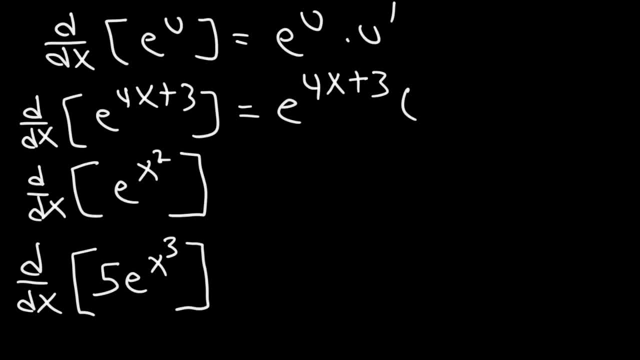 e to the 4x plus 3, and then times the derivative of 4x plus 3, which is just 4.. So it's 4e to the 4x plus 3.. Now for the second one. it's going to be the same thing. 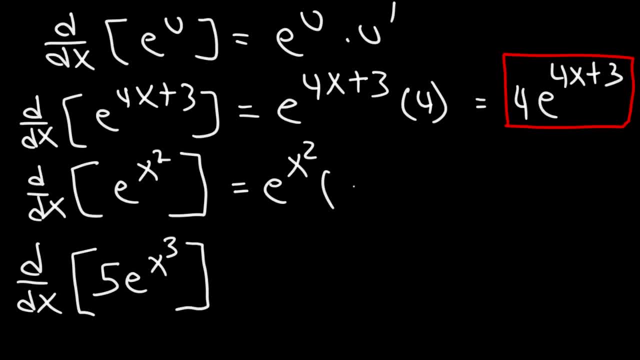 e to the x squared, times, the derivative of x squared, which is 2x, And so it's 2x. e to the x squared. And for the last one, it's going to be what we started with: times, the derivative of x cubed, which is 3x squared. 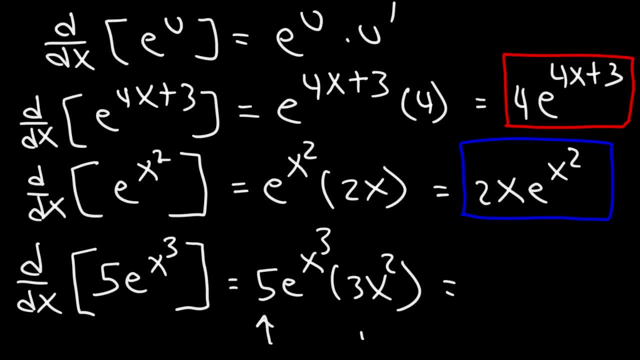 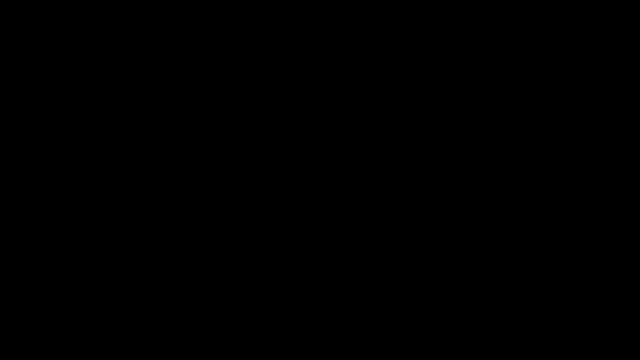 And so we can multiply 5 and 3.. And that's going to give us 15x squared e to the x cubed. And so now you know how to find the derivative of exponential functions with the base e. Next let's talk about finding the derivative of logarithmic functions, particularly the natural log function. 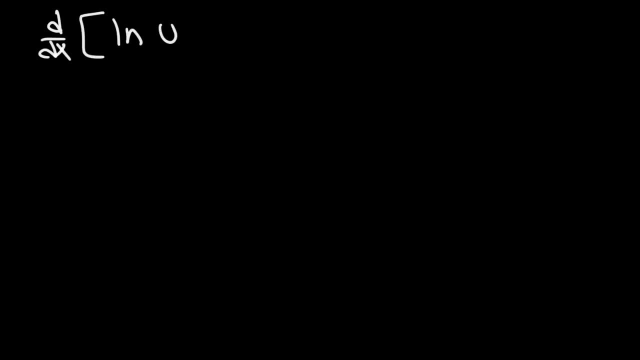 The derivative of ln- u, where u is once again a function of x, is u prime divided by u. So let's say: if we want to find the derivative of ln- x, So in this case u is x, u prime, the derivative of x is 1.. 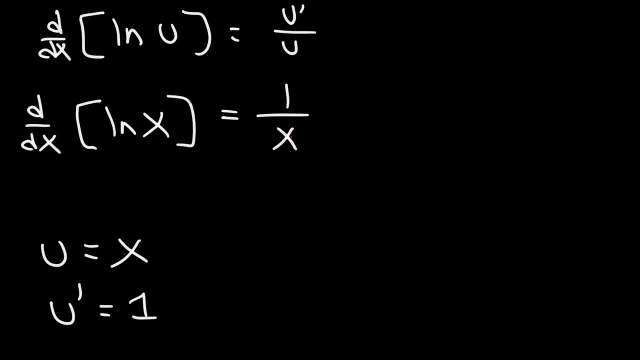 So u prime is 1, u is x. so the answer is just 1 over x. Let's try another example. Let's find the derivative. Let's find the derivative of the natural log of x squared plus 5.. So u is, that's the stuff inside the natural log. 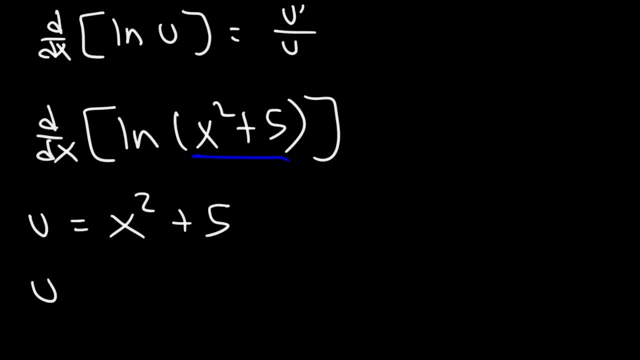 That's x squared plus 5.. u prime, the derivative of x squared plus 5, is just 2x, So it's going to be u prime divided by u, And so the answer is 2x over x squared plus 5.. 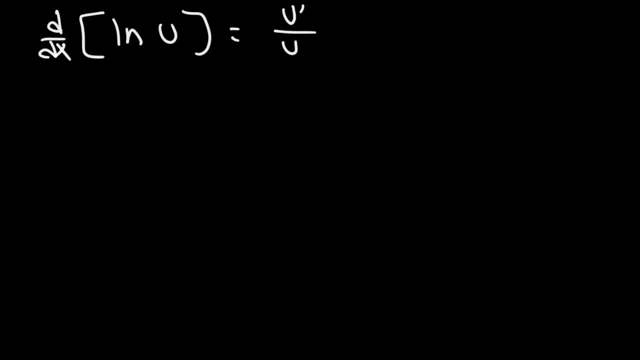 For the sake of practice, try this one. Find the derivative of 3 times the natural log of 5x plus 4.. So u, the u variable is going to be 5x plus 4.. And u prime is the derivative of 5x plus 4.. 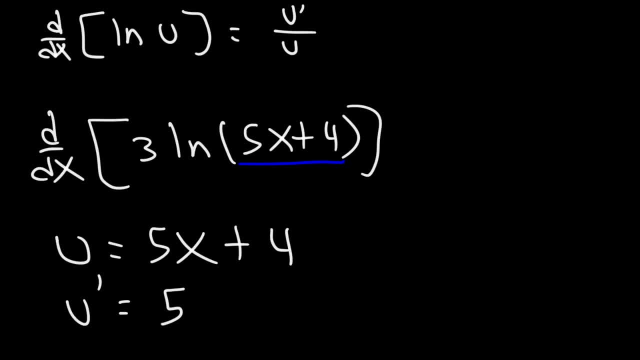 The derivative of 5x plus 4 is u. The derivative of 5x plus 4 is u, 5x is 5, and the derivative of the constant 4 is 0, so it's just 5.. Now we do have a constant in front of the natural log, so we're going to rewrite that here. 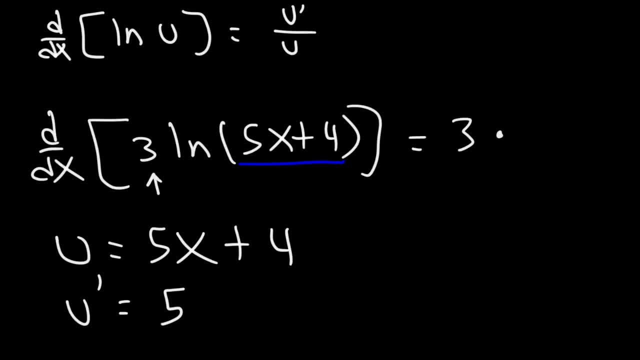 So it's going to be 3 times this thing: u prime, which is 5, divided by u, which is 5x plus 4.. So now we can multiply 3 times 5, and that's going to be 15.. 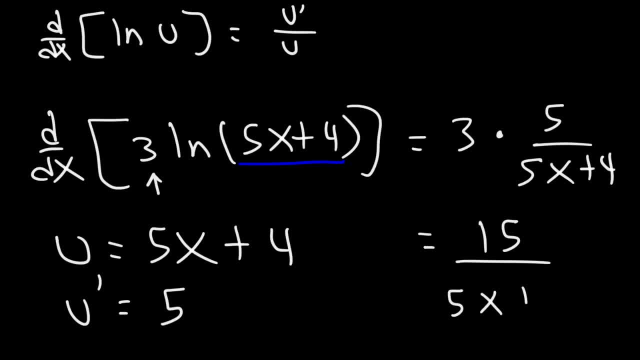 So the answer is 15 over 5x plus 4.. So now you know how to find the derivative of natural logarithmic functions. Now for those of you who want more example problems on not just natural logs but logarithmic functions, exponential functions and other things like implicit differentiation and things like that. 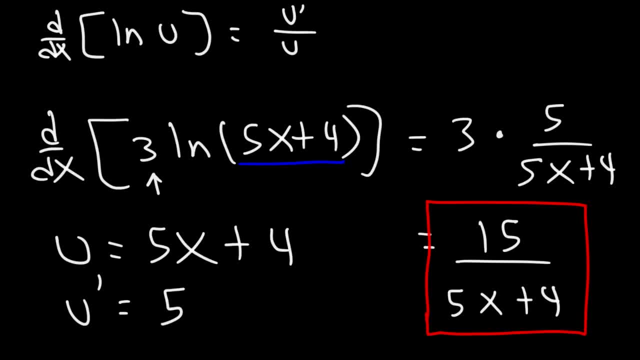 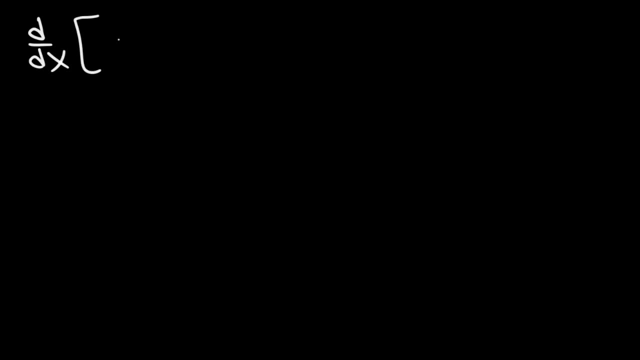 check out the links in the description section below, And I'm going to post more videos, And I'm going to post more video resources that can help you with derivatives. Now the next thing we need to talk about is the product rule. The best time to use the product rule is when you have two things multiplied to each other. 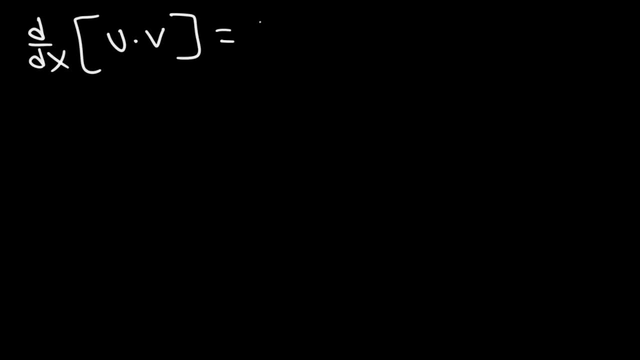 Let's say u and v. So what you need to do is you need to differentiate one of these two functions. So if you differentiate, u first leave the other one, And then it's going to be plus. We're going to leave the first function the way it is and differentiate the second one. 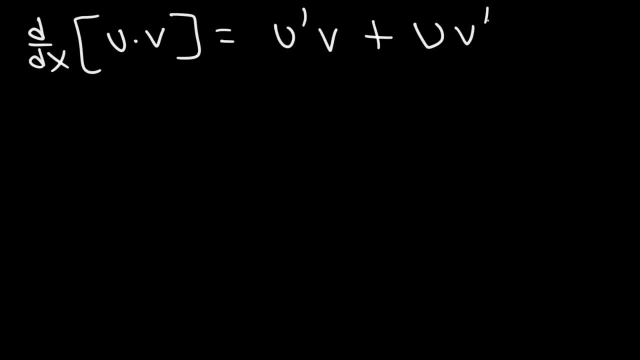 So the derivative of u times v is going to be u prime v plus u v prime. I need to draw the u better. So this is a u, that's a v. Now let's work on some examples. What is the derivative of x squared times sine of? 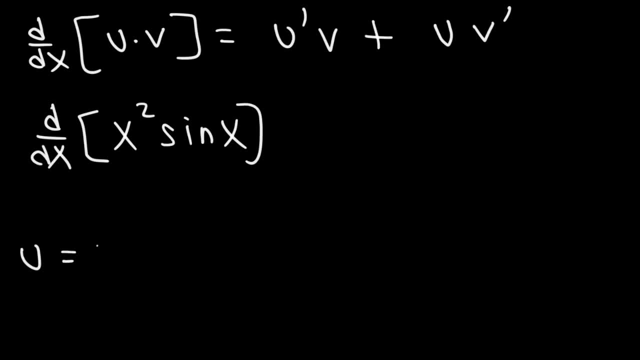 So in this case u is x squared, which means u prime is 2x. v is going to be sine x, So v prime is cosine x, So it's going to be u prime times v plus u times v prime, which is cosine.